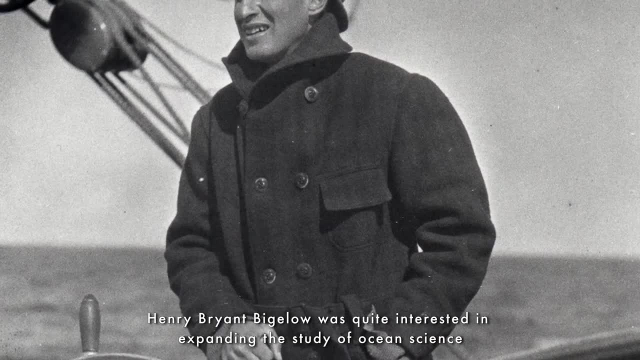 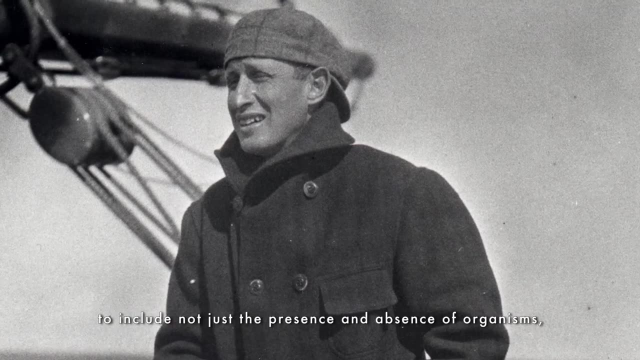 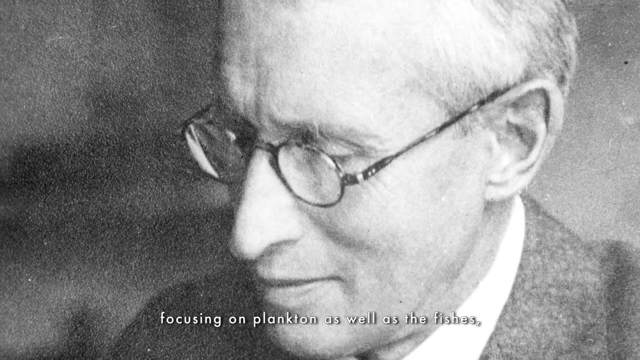 Henry Bryant Bigelow was quite interested in expanding the study of ocean science to include not just the presence and absence of organisms, but measurements of physical and chemical properties, focusing on plankton as well as the fishes, realizing that it was the cycle of plankton production in the Gulf of Maine that 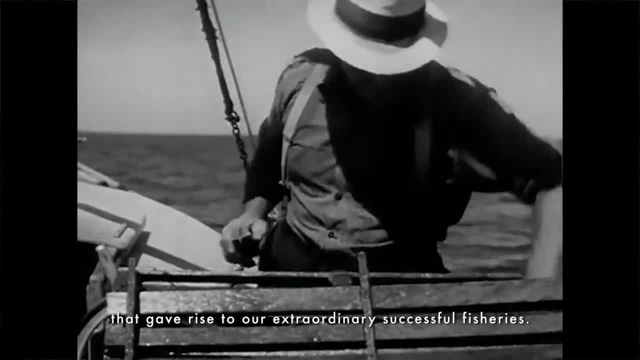 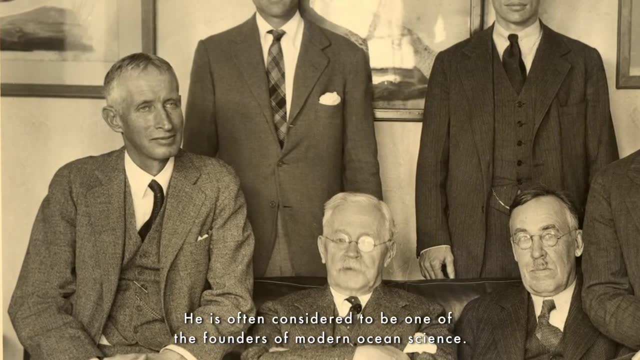 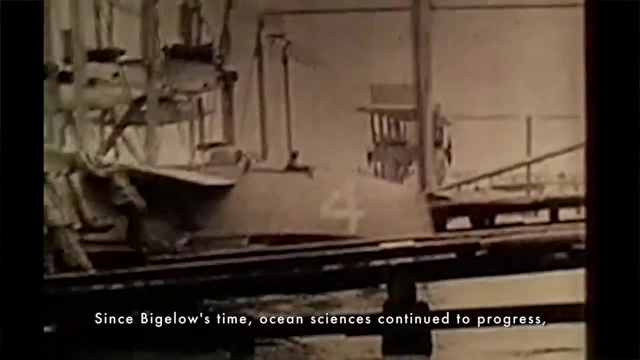 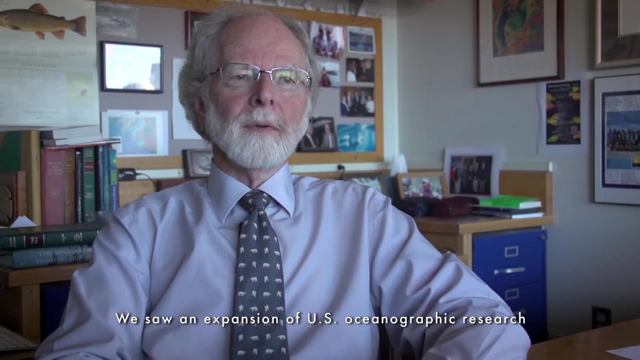 gave rise to our extraordinarily successful fisheries. He is often considered to be really one of the founders of modern ocean science. Since Bigelow's time, ocean science has continued to progress, in part with the development of new technologies. We saw an expansion of US oceanographic research. 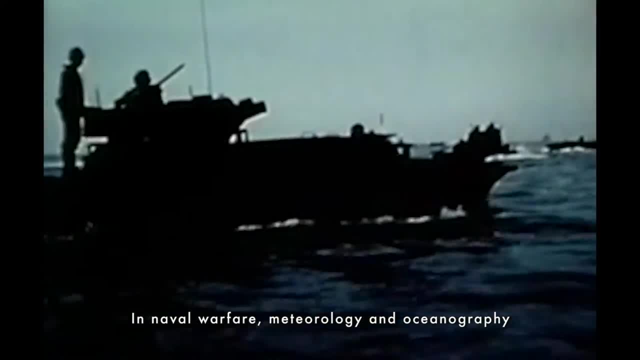 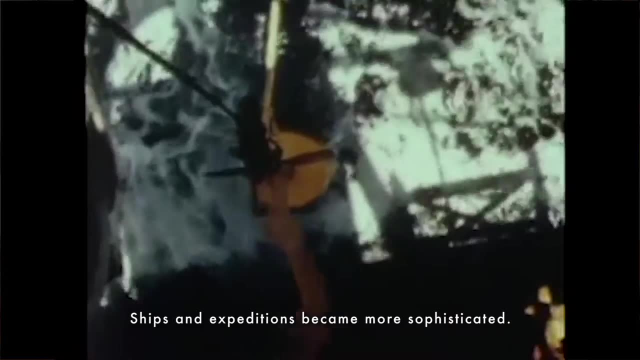 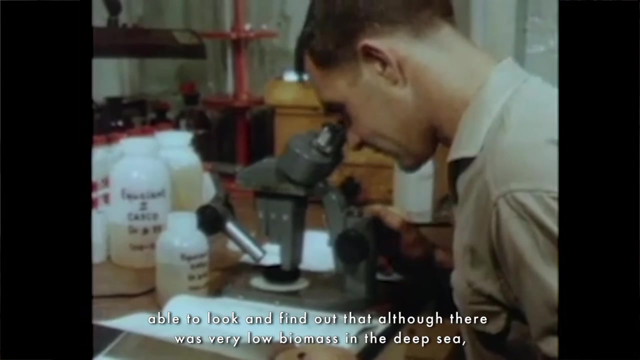 following World War II. In naval warfare, meteorology and oceanography must be considered as one discipline. Ships and expeditions became more sophisticated. They were able to retrieve sediments, able to look and find out that although there was very low biomass, there was very little life in the deep sea. It was extremely diverse, But basically there's not much food in the deep sea, so nothing, you know, they were thought to just be spars. In 1960, with the dive of the Bathyscaphe Trieste into the Mariana Trench, 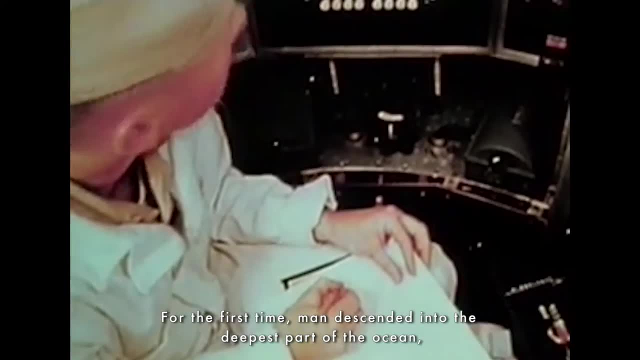 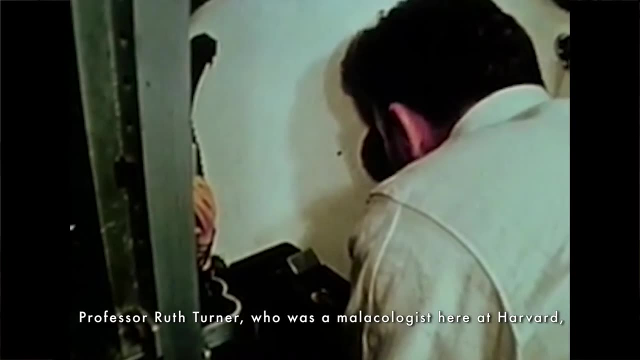 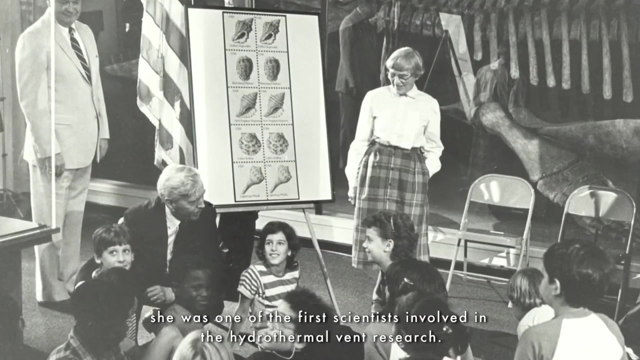 a new era in deep sea research began. For the first time, man descended into the deepest part of the ocean nearly seven miles down Professor Ruth Turner, who was a malacologist here at Harvard. she was one of the first scientists involved in the. 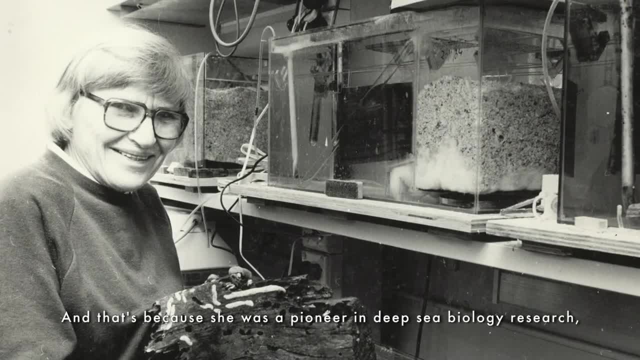 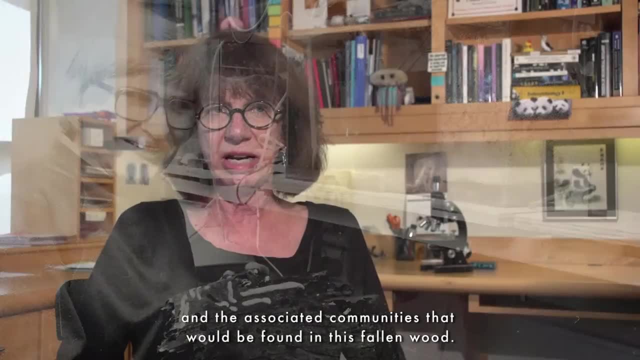 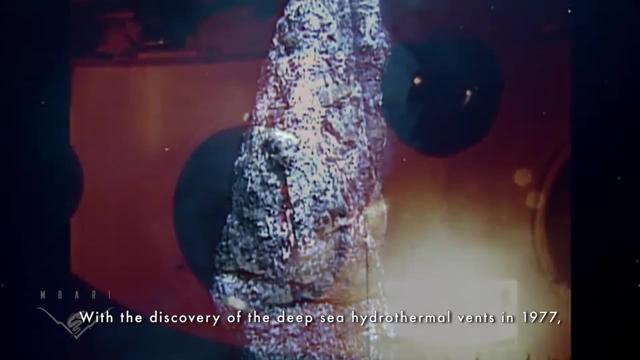 hydrothermal vent research, And that's because she was a pioneer in deep sea biology research, focusing primarily on shipworms, which are actually bivalves, and the associated communities that would be found in this fallen wood. With the discovery of the deep sea hydrothermal vents in 1977,. 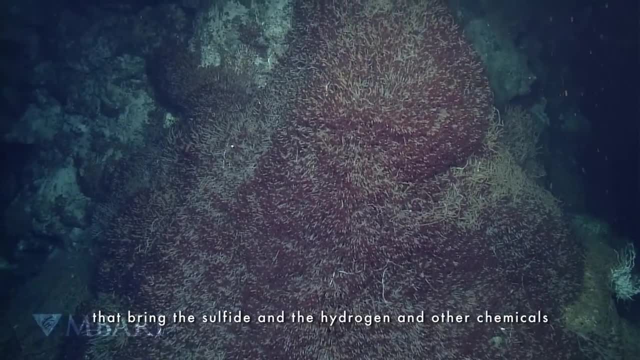 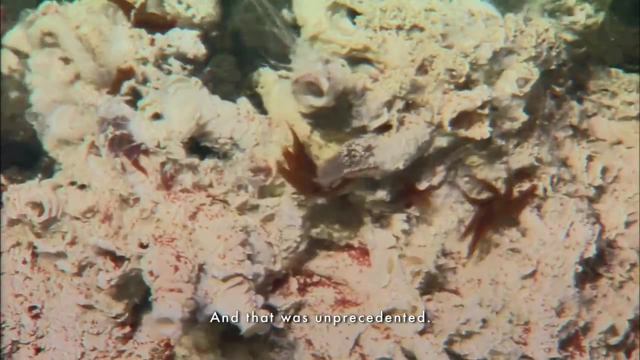 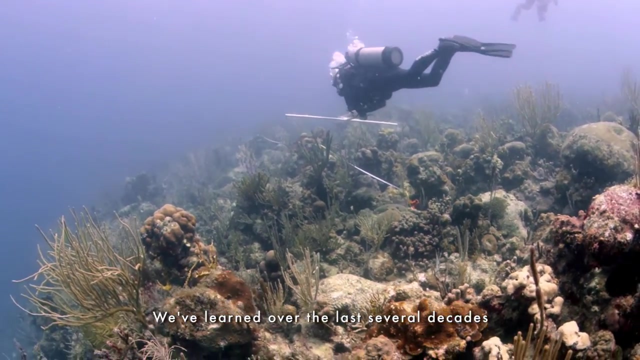 these are oases of animals surrounding these warm vents bring the sulfide and the hydrogen and other chemicals that bacteria live on. that then feed the ecosystem, And that was unprecedented. We've learned over the last several decades that it's the life processes in the ocean. 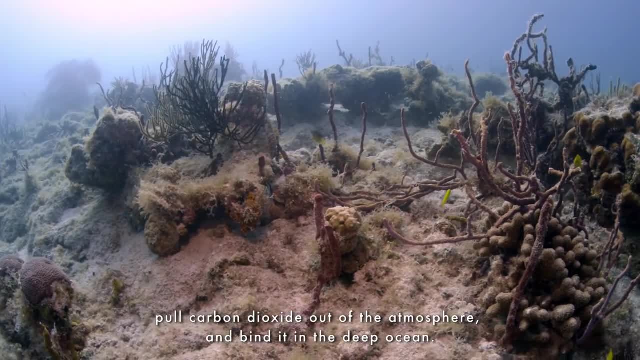 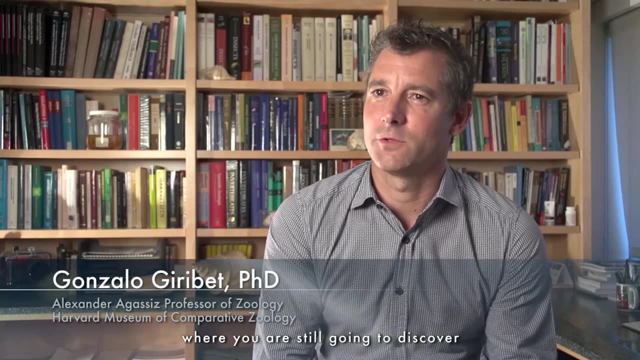 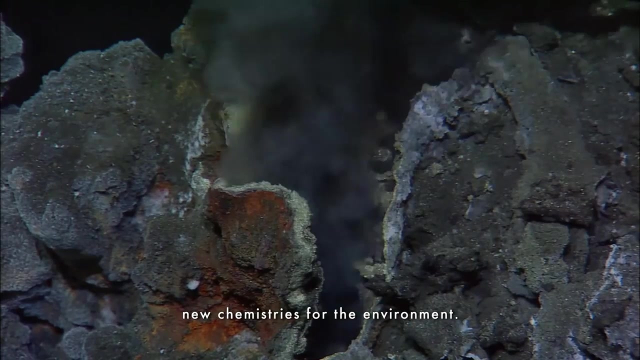 that, over the long run, pull carbon dioxide out of the atmosphere and bind it in the deep ocean. This is the only place in the planet where you're still going to discover very large animals, new forms of life, new chemistries for the environment.